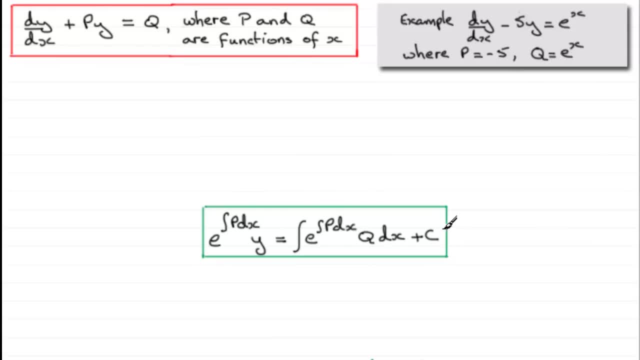 Maybe a bit horrendous at this stage, but using it generally isn't too bad, As I demonstrate. if you were to click on this link here, it will take you through the solution to this, But if you go on my website, examsolutionsnet, you'll see more links to other examples that are similar to this. 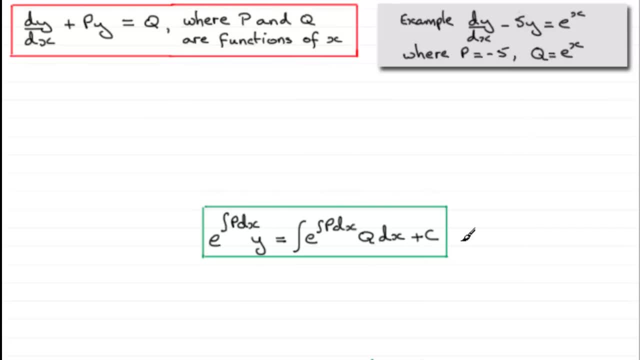 Now, the object of this video is to show you how we derive this equation. It's not something you might necessarily need to be able to prove, but nonetheless I'll take you through it. But certainly try and learn this particular equation so that you can apply it in situations like this. 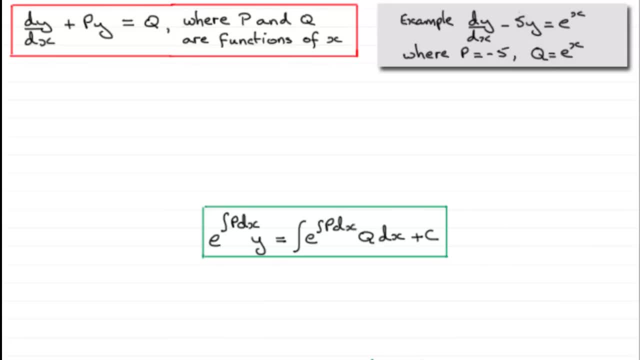 Okay. so what we'll do is we'll just remove this for the time being And we'll start with a general equation. then Let's say that we will just copy this down. Okay, Anyway, let's say so. if we have dy by dx- okay- plus py equals q, then what I'm going to do is multiply throughout by some function of x. 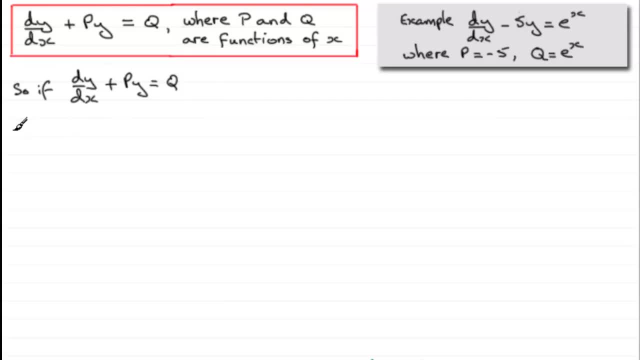 Okay, We'll just call it f of x. So what I'll say here is: we'll multiply, Okay, Both sides of our equation, okay, by some function of x. And the reason for doing this is it turns it into what we call an exact differential equation. 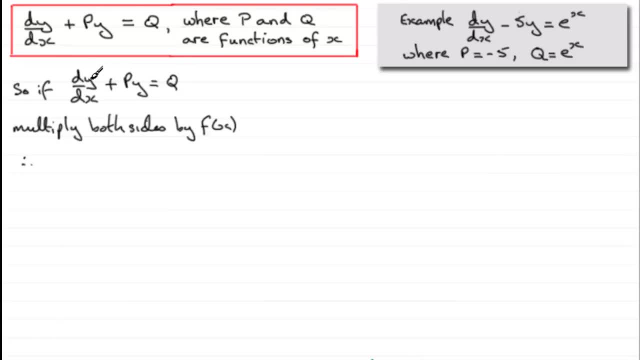 So if we do that, we'll have f of x times dy by dx, f of x multiplied by dy by dx, And then we would have f of x times dy by dx. Okay, f of x, py, And then next we'd have f of x times q. 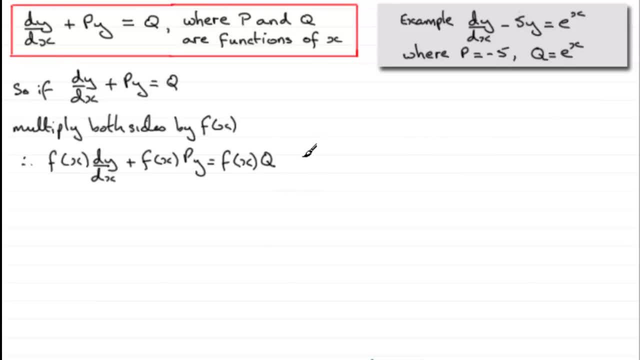 Now, the reason for doing this, as I said, was to turn it into an exact differential equation. I'll call this line here one, as you can see, And by that I mean that if we were to differentiate, I'll just say: but. 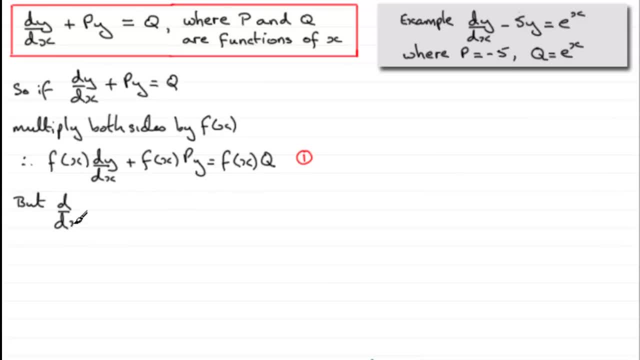 Okay, Okay. If we were to differentiate with respect to x, say this particular function f of x multiplied by y, what would we get? Well, we'd need to use the product rule for something like this. In other words, we'd write down: say f of x. 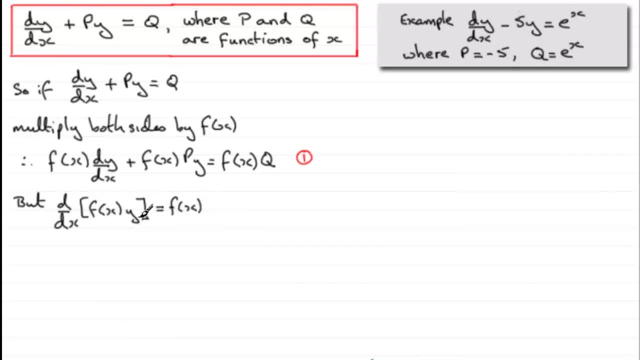 And then we would multiply it by the differential of y with respect to x, In other words, that's dy by dx. And then we would add to that the differential of f of x with respect to x, which would write as f dash x or f prime x. 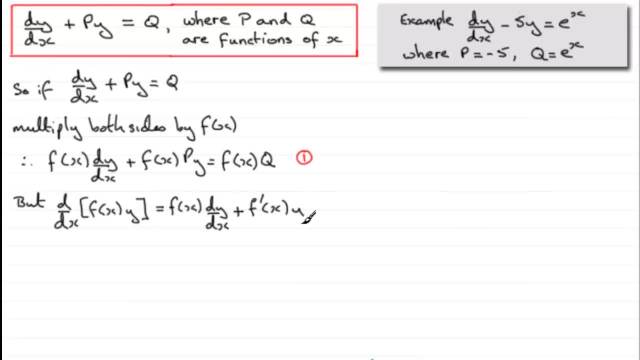 And we would multiply that by y. So that's the product rule. then Let's number this equation here too. Now, if I compare the left-hand side LHS of equation y of equation 1, with the right-hand side RHS of equation 2,, 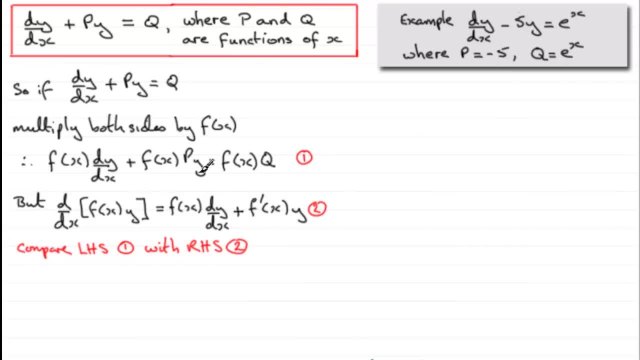 then I notice that there is some similarity. If we just copy down the left-hand side of 1,, we've got f of x multiplied by dy, by dx plus, and then we've got f of x- py. Let's just write the f of x p. 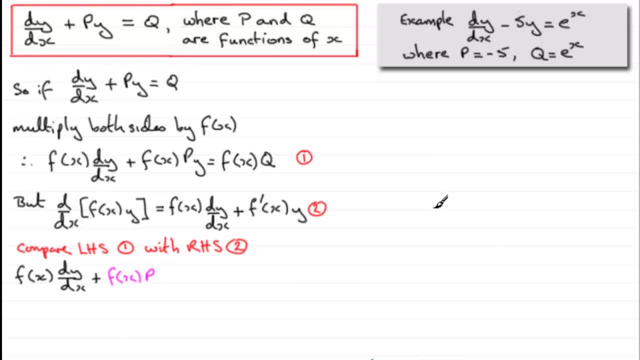 in this colour, f of x, p, And then we've got the y, And this is identical to the right-hand side of equation 2.. In other words, we've got f of x again multiplied by dy, by dx. 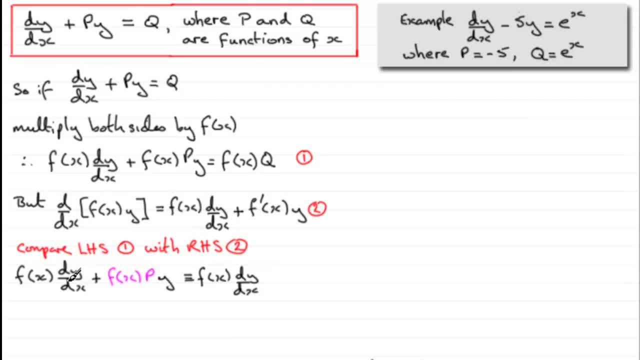 So the first two terms are exactly the same, And the second term is a term with y in, but we've got the f dash x. So let's just put f dash x in this colour, and then we'll put the y in. 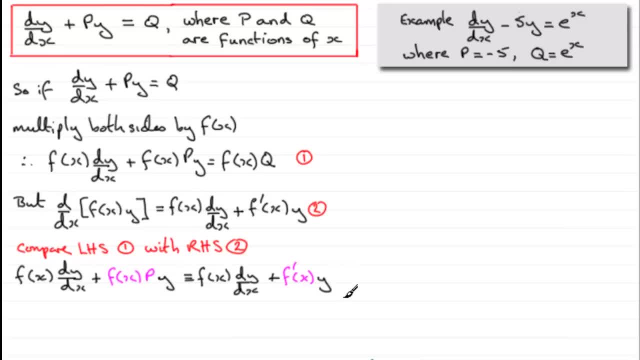 So hopefully you can see the terms match up. So what I see now is that f of x, p must be exactly the same then as f dash x, And if I now divide both sides by f of x, I get that therefore, f dash x over f of x. 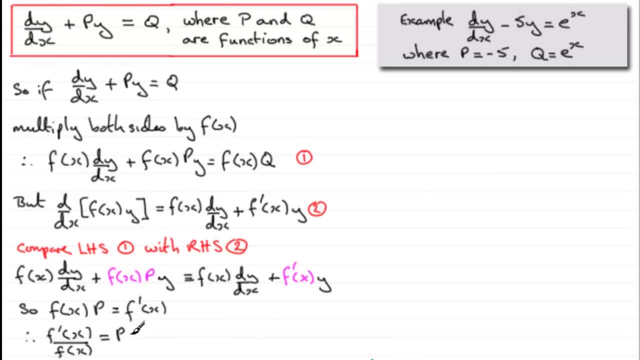 must be equal to p, And if I integrate both sides with respect to x, it follows then that the integral of f dash x, all divided by f of x, and if this is integrated with respect to x, it must be equal to the integral of p with respect to x. 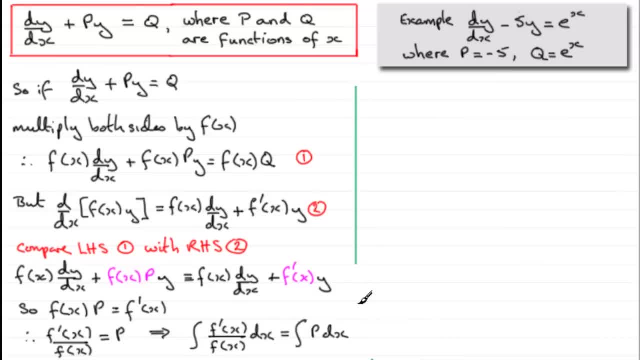 Now, if we just come down here Now, this type of integral should be familiar. where we have f dash x over f of x, It is the natural log of the denominator. So therefore we have the natural log of the mod of f of x. 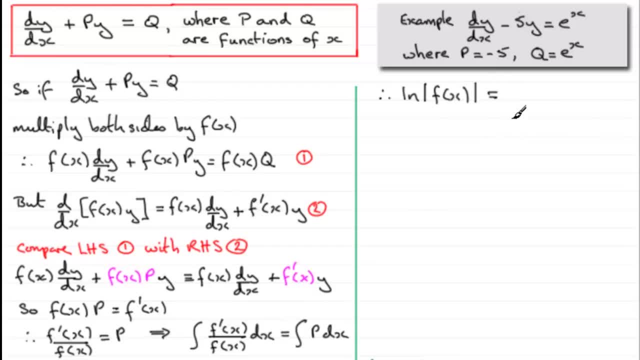 is equal to the integral of p with respect to x. Now, if I antilog this, I therefore have that f of x must be equal to e, to the power, the integral of p with respect to x, And we'll label this equation 3.. 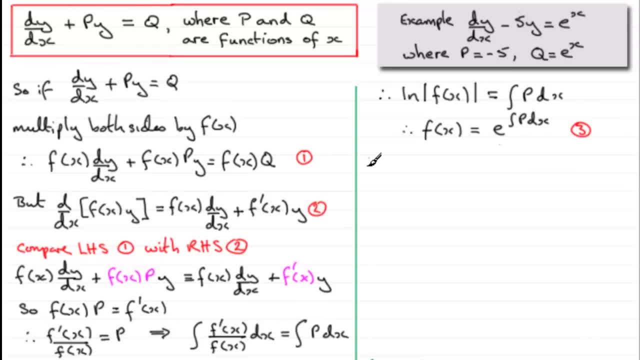 Now e to the integral p. dx is often referred to as an integrating factor. You'll see this cropping up a lot in any solution, So we'll just mark this in. So it's called the integrating factor. Okay, integrating factor. Now, if we return back to equation 2,, 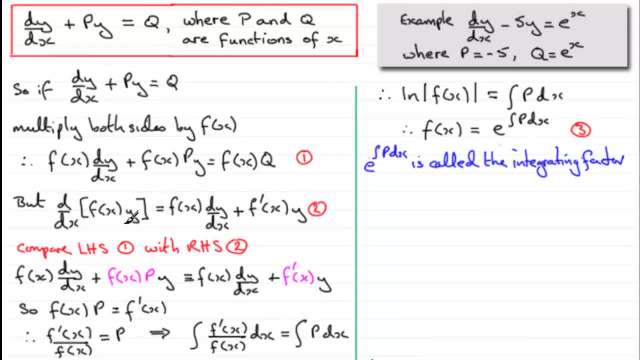 if I was to substitute the left hand side of the equation into equation 1, remember I've shown you that this is identical to this. So in other words, I can write that the differential with respect to x of f of x, y must be equal then to f of x times q. 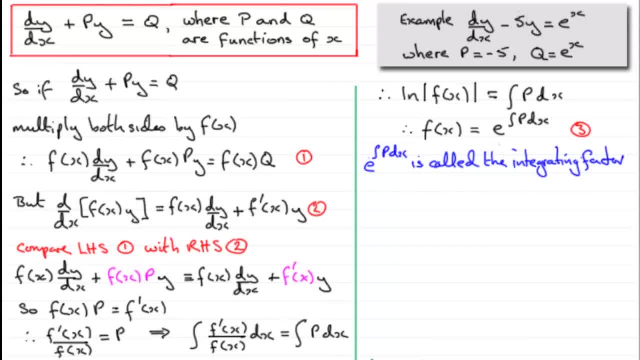 So if I was just to substitute that in, let's just write this in here: substitute the left hand side LHS of equation 2 into the left hand side of equation 1, then what we have got is that the differential with respect to x of f of x times y. 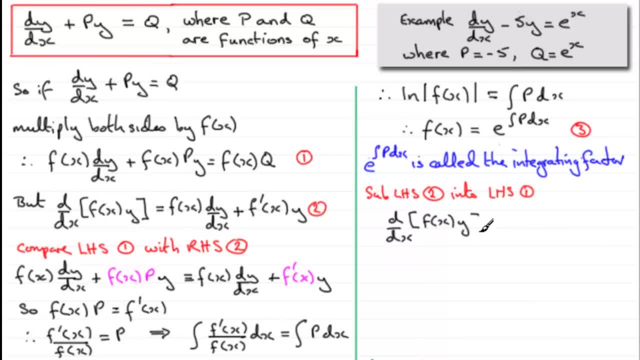 f of x multiplied by y must be equal to f of x times q, f of x times q. Now that means that if I integrate both sides with respect to x, I therefore have f of x multiplied by multiplied by y. okay, equals the integral of the right hand side with respect to x. 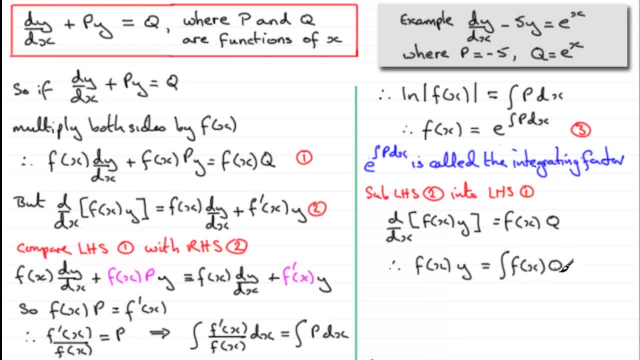 the integral, in other words, of f of x times q integrated with respect to x. And now we can see that from equation 3, f of x is equal to e, to the integral pdx, the integrating factor, in other words. So if we just say that, 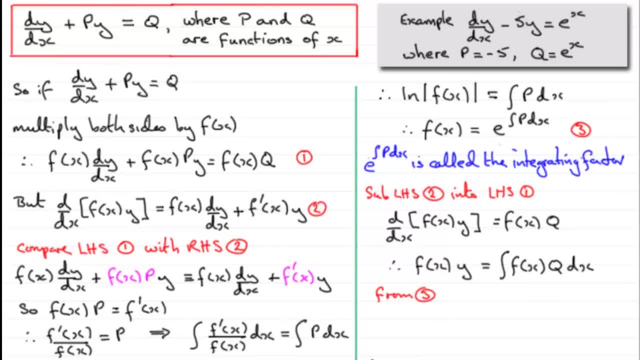 from 3, what we therefore get is that f of x, which is now e, to the integral pdx. so we have e to the integral pdx. f of x is now multiplied by y and it equals the integral of f of x. 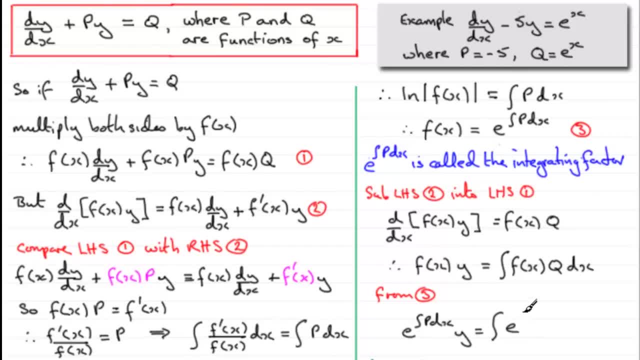 which is the integrating factor. again e to the integral pdx multiplied by q, And this is integrated with respect to x. And don't forget, we would have a constant of integration, let's say plus c. So this is known as the general solution.